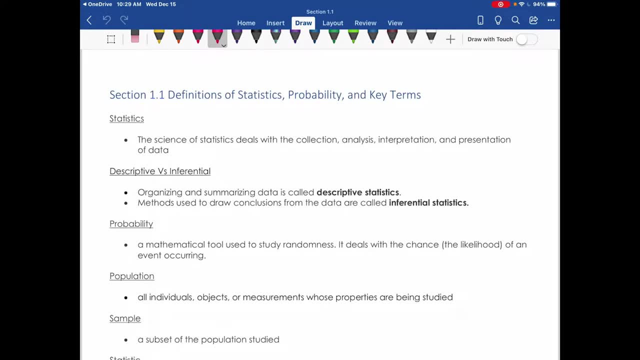 Welcome to statistics class. This is our first lesson in section 1.1 of the OpenStax textbook And in this section I'm going to go over some key concepts in terminology with you to get us started in the class. So, overall, the idea of statistics as a course or a path of study- because there's another definition on statistics that I'm going to talk to you about here in a minute. 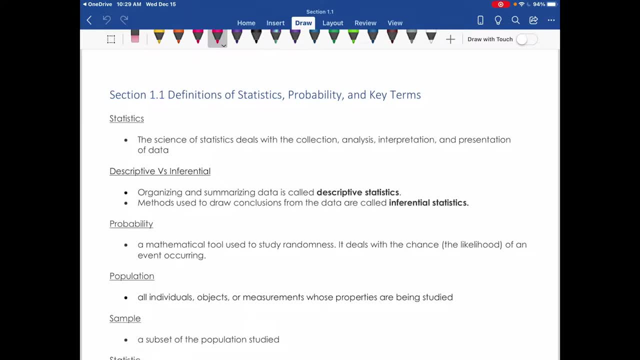 But the statistics. when we talk about a statistics course or studying statistics is the science of collecting and organizing, analyzing and interpreting data in order to get us started in the course, In order to make decisions. Now, there are two branches of statistics and you'll see them listed here. 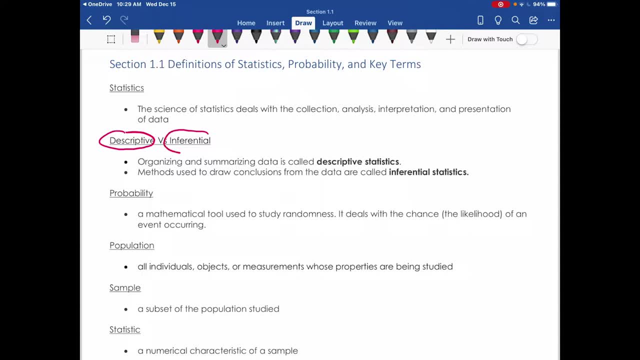 There's descriptive and then there's inferential. When we talk about descriptive statistics, we're talking about the branch of statistics when you collect data and then you organize it and you summarize it, usually in tables and charts and histograms and those kinds. 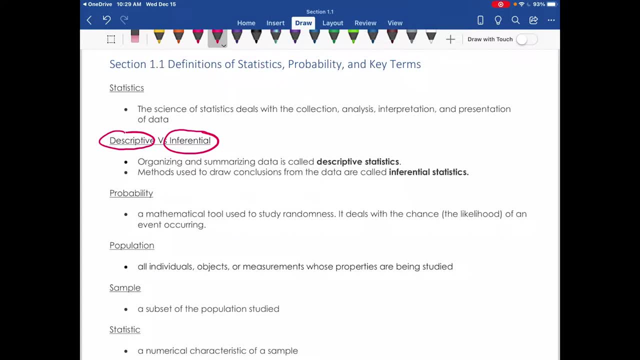 So when you're organizing and summarizing the data, that's called descriptive statistics- But then when you want to go to make your decisions and draw your conclusions, you have to use mathematical techniques in order to do that. Now, those formal methods. when we go through that process of those formal methods to draw our conclusions and come up with our decisions, 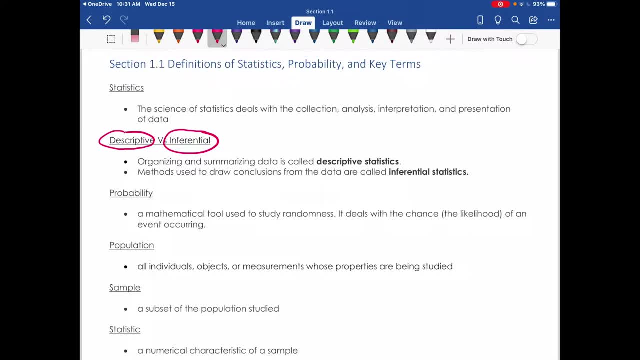 that branch of statistics is called. The next term we're going to talk about is probability. Probability is a mathematical tool used to study randomness and it deals with the chance or likelihood of an event occurring. Now, probability is a big part of statistics because when we get into the branch of statistics, where we are using formalized methods to draw conclusions, 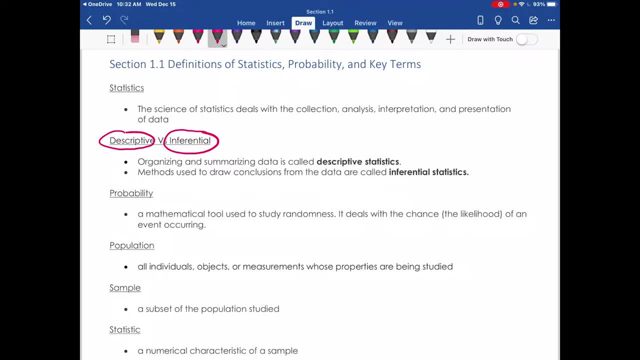 which is that inferential branch of statistics. we use probability to help us make our decisions, So probability is integrated quite a bit in that second branch. There are two data sets that we're going to really focus on, That is, the population, and I'm going to color code this to help you see what's going on here. 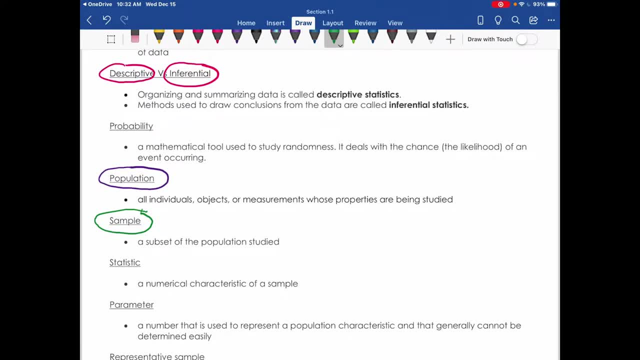 There's the population, which is a data set, And then there's the sample, Which is a data set. Now, the population is the collection of all the individuals or all the objects and measurements that you're trying to study. Whatever it is that you're doing research on, that you're trying to find out about. 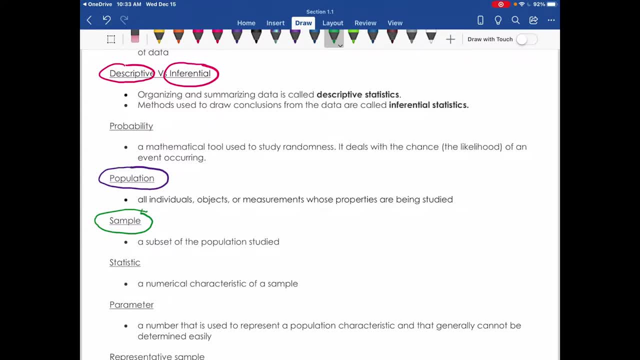 the population is the data set that encompasses all those people or all those objects that you're trying to find out about. So when you take a sample, that is a subset where you pull out of the population, a subset of the population, So it's a smaller set that comes out directly from the population. 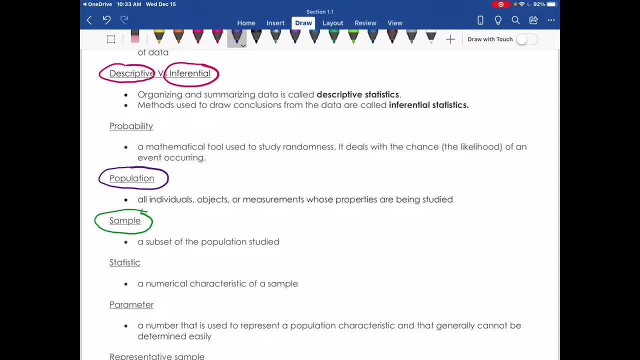 So if you think of the population, of everybody that you want to study about, or everything that you want to study about, is inside this circle, And so the population includes all of these things inside the circle, When I pull a sample out, a lot of times it's impossible to find all the people or all the things that you're trying to research. 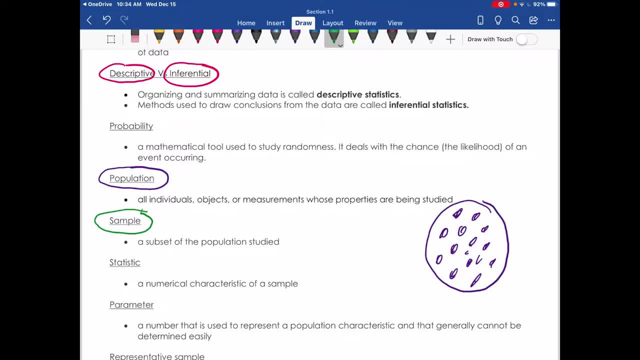 Most of the time that's completely unrealistic. So you take a sample of that and use the sample to draw conclusions. So a sample would be if I just select certain ones out of the population and use that to find my calculations and to form my opinions and interpretations and estimations. 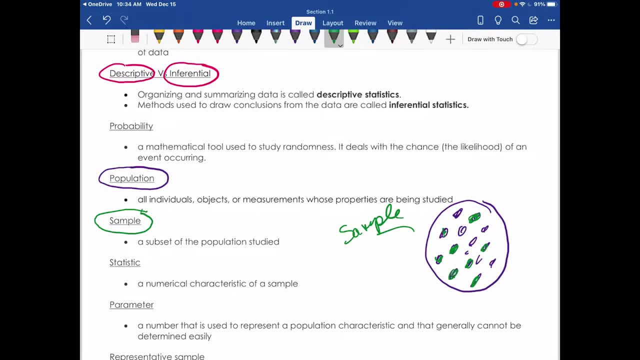 So the sample is specifically used to gain information about the population when you can't, when you don't have access to the entire population. Now, when I create my sample, when I come up with the value that represents that sample, maybe I'm trying to find the average of something or a proportion of something. 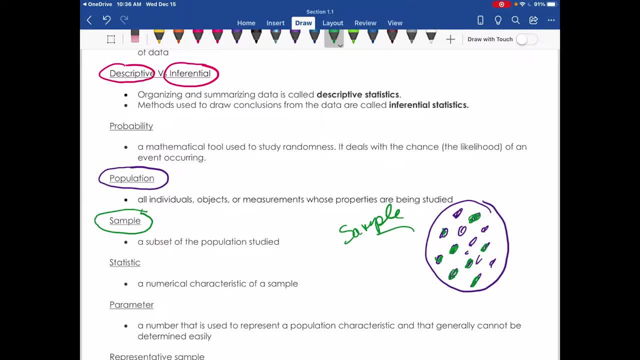 That value that I get from the sample is called a statistic. That's this here. A statistic is a numerical characteristic of a sample, which is a fancy way of saying a number. numerical characteristic, a number that represents the sample. It could be a mean or an average. 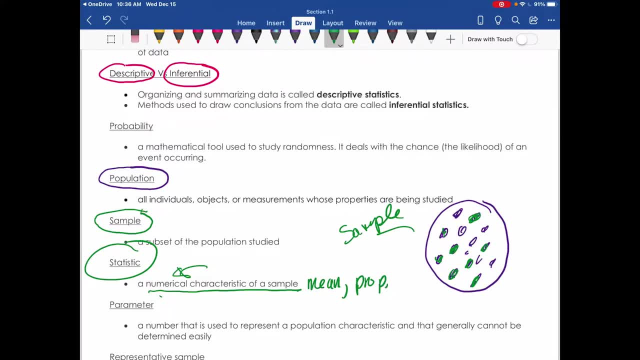 It could be a proportion. So when I make those calculations based on the sample- because the population is too big to try to make those calculations on the entire population- that number that I get from the sample is called a statistic, And that's why I'm highlighting these two in green. 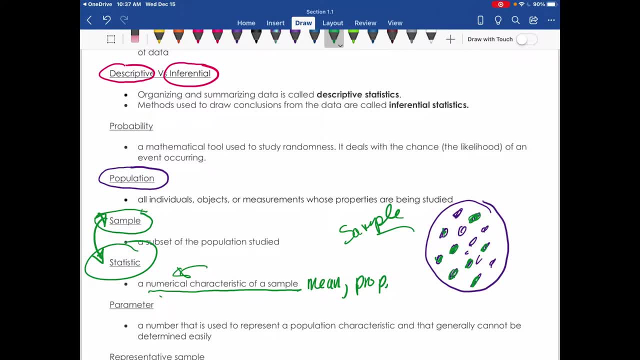 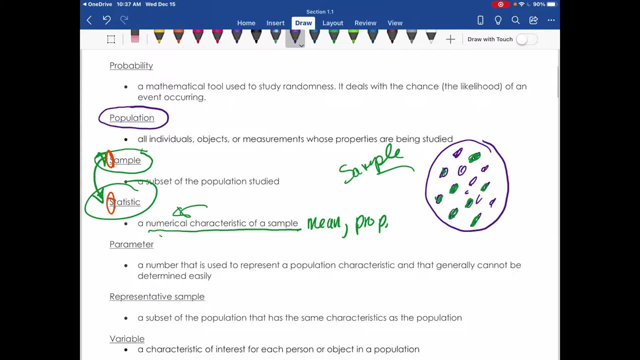 The statistic comes from the sample And another way that I always remembered it when I was learning this for the first time: S and S. So statistic goes with sample. Now that same idea goes with parameter. If for some reason I was able to get in touch with every American, 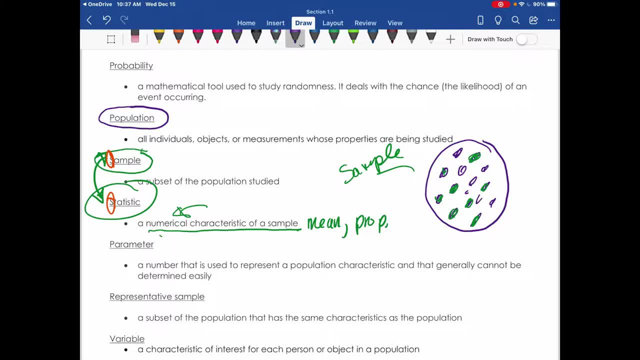 okay, and whatever it is that I'm trying to find out, maybe I'm trying to find the average height of all Americans, If, for some reason, I am able to get in touch with all Americans and I calculate the average height of all those people. 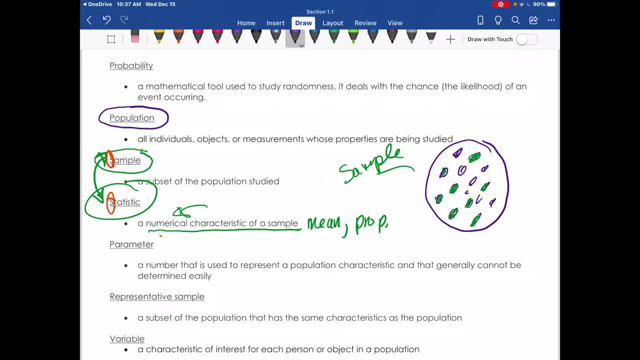 then the number that represents the population, that average that I calculate from everybody, is going to be a parameter, because the parameter is a number that represents a population characteristic. So the parameter comes from the population And again, here's a way to remember it. 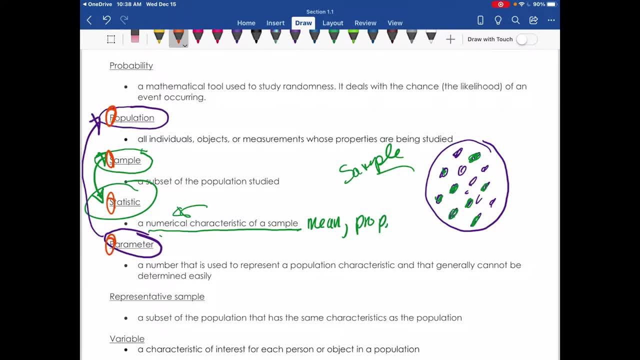 P and P. population and parameter Parameter comes from the population, So statistic and a parameter. those are numbers. They could be averages, proportions, It could be a mean, It could be a standard deviation. Any number that represents a population is a parameter. 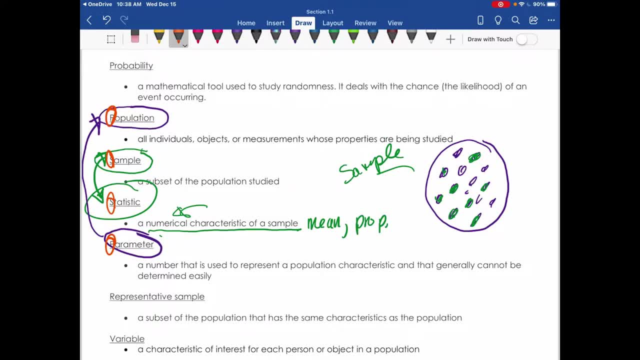 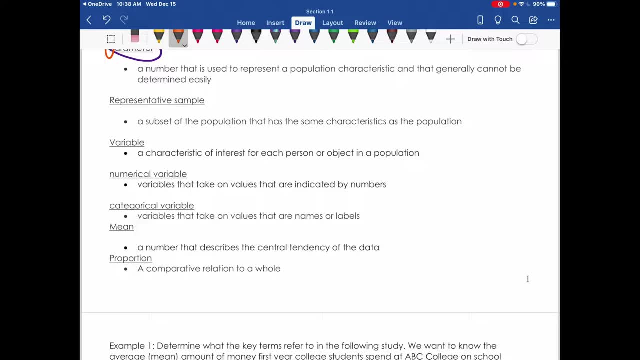 And numbers that represent samples are statistics. Now, when you take a sample, you want to make sure that you get what's called a representative sample And that is a subset of the population that has the same characteristics as the population. Now, a variable is a characteristic of interest. 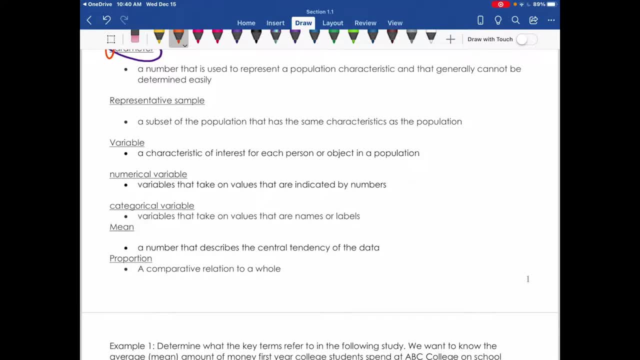 for each person or object in a population. So a variable is going to represent whatever it is that you're trying to measure. So let me put that in parentheses. So, for example, if I was doing a research project where I was trying to find the average height of Rogue State students, 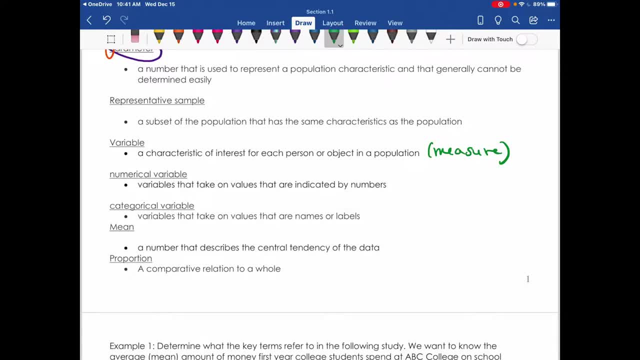 I would go around and I would find a sample of students and I would ask each of them their height And then I would average those values together. Well, when I go and approach each student and ask them their height, that height is going to change from person to person. 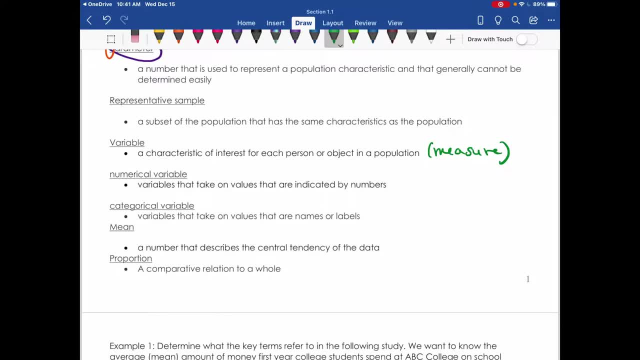 So the height is going to be the variable. It's what I'm measuring and what is going to change from person to person in that situation. Now, a numerical variable are variables that take on values that are indicated by numbers. Then you have categorical variables. 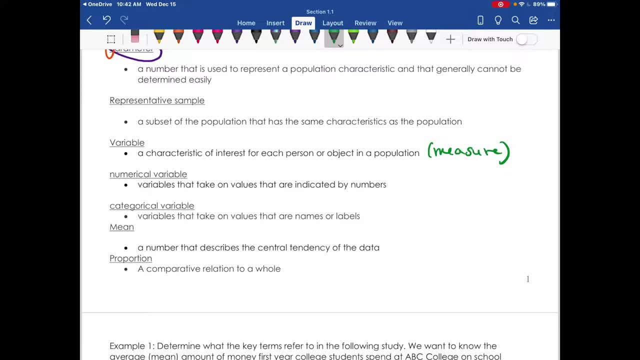 that take on values, that are names or labels. So, for example, if I was trying to do a study on how many people have red cars or how many people have blue cars, the variable would be the color, because when I approach each person to find out what color car they have, 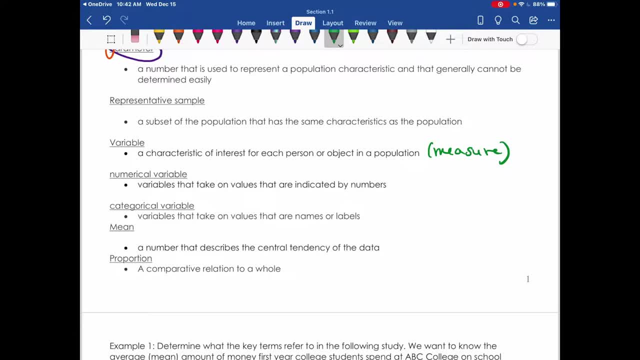 it's going to change. The color is going to change from person to person. So that's going to be my variable: the color of the car. And the variable is not a number, It's going to be a color. It's going to fall into a category. 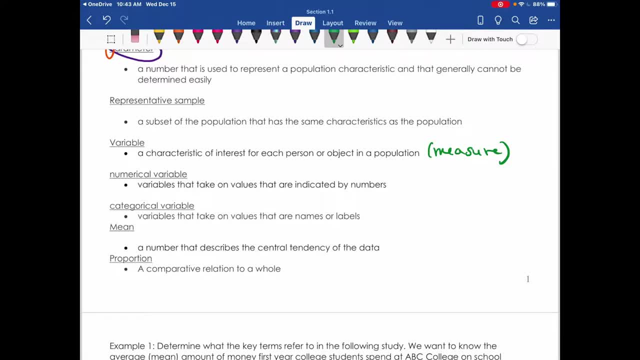 By using a name or a label. So that's an example of a categorical variable. Now, your mean is the number that describes the central tendency of the data. That's going to indicate an average of the data. The mean is the average that we're familiar with. 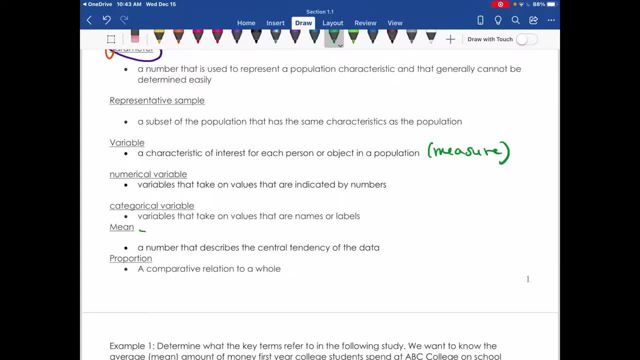 There's different kinds of averages. The average that we're familiar with is when you add all the values and you divide by the number of values that you have. That's the mean. We'll get into other kinds of averages later on. A proportion is a comparative relation to a whole. 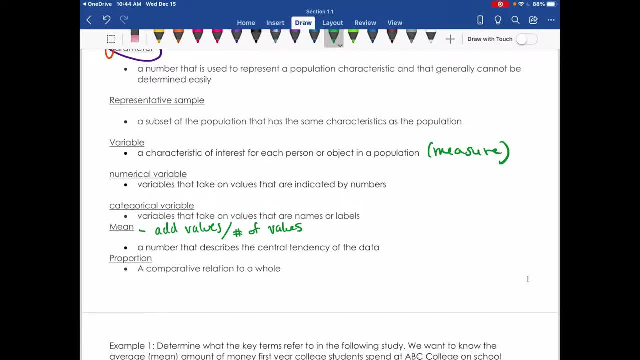 So if I was comparing how many people out of a total had red cars, for example, that might be a proportion of. I'm just going to make sure I make up a number here, Say 35 out of 100. And that could also be written as a percentage. 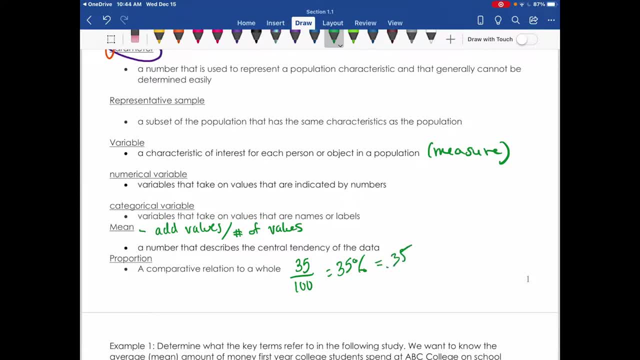 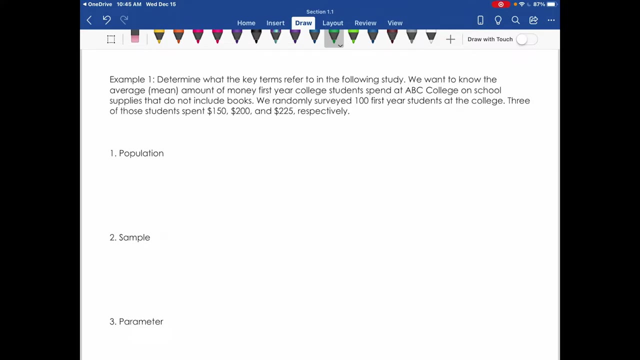 or as a decimal. So you're comparing the amount to a whole. So that's your proportion. Now let's go through the first example And we're going to go through some of these major terms and identify them. Okay, 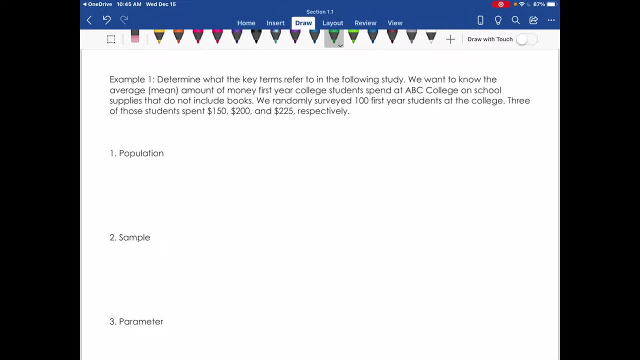 We're going to determine the key terms that refer to the following study. We want to know the average or the mean amount of money first-year colleges spend at ABC College on school supplies that do not include books. We randomly surveyed 100 first-year students at the college. 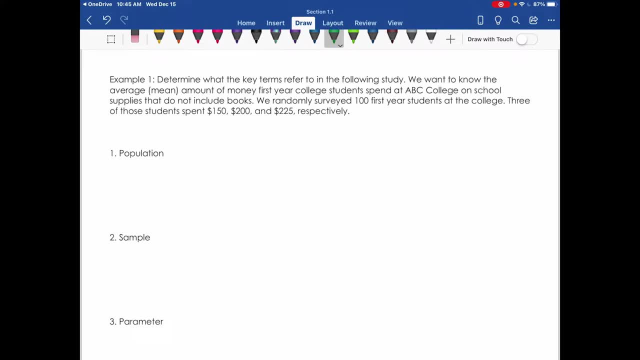 Three of those students spent $150,, $200, and $225, respectively. So when you're identifying the population, it's really important to go back after you read the question or the situation through one time to get an idea of the topic. 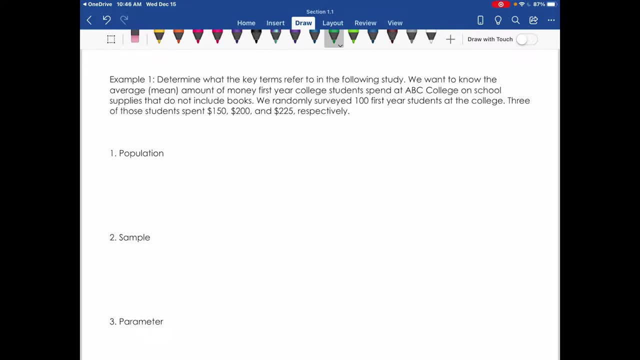 It's really good to go back and look at the wording, because one word can change everything, the whole meaning. So when you first think about the population, you're like, oh well, this person is doing a study on college students. 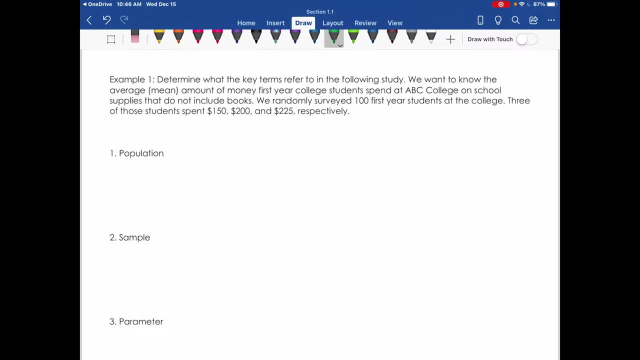 So I would put down in the population all college students at ABC College. When you go back and look at the wording, being very careful, specifically they're looking at first-year college students. So I highly recommend to not just jot something down very quickly. 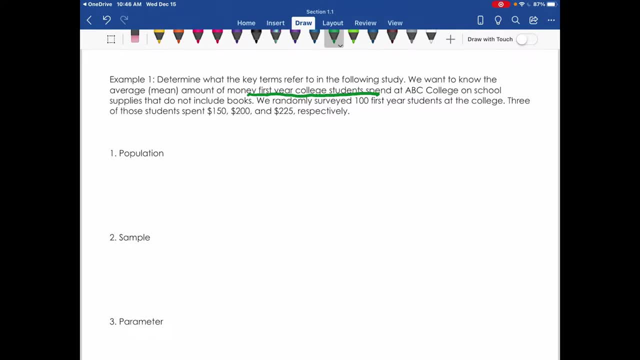 to really go back and underline what the key words are in the question, to verify that you are identifying the correct population. For another example that you might make a mistake on, just to throw this out there, you might quickly read about a survey given to Americans that are over 65,. 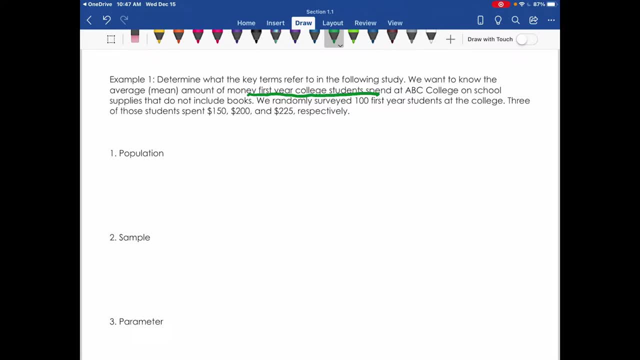 senior citizens. And so you might think, oh, the population is all Americans, because they're doing a survey, they're giving a survey to Americans, But when you read the problem carefully, they're specifically identifying senior citizens. So you want to say: 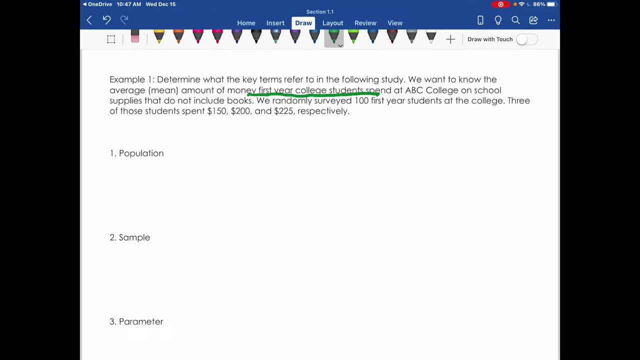 all senior citizens in America. That would be your population. So be very careful and go back and underline to make sure that you are identifying the correct population. So for this population I would put all first-year students at ABC College- Another mistake you might make. 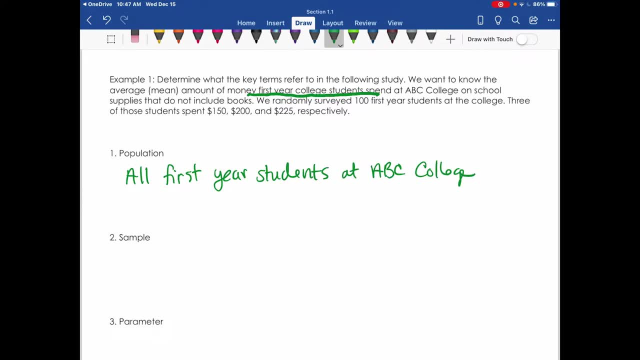 is, you might put down all first-year students. That's not true, because just with this change right here, just that word change, that means something completely different. They're only looking at first-year students at this college, this ABC College. So don't put down. 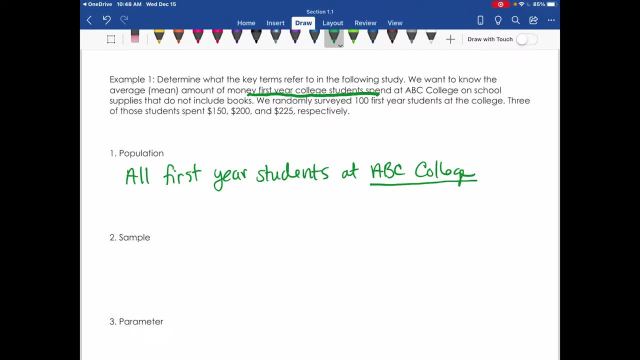 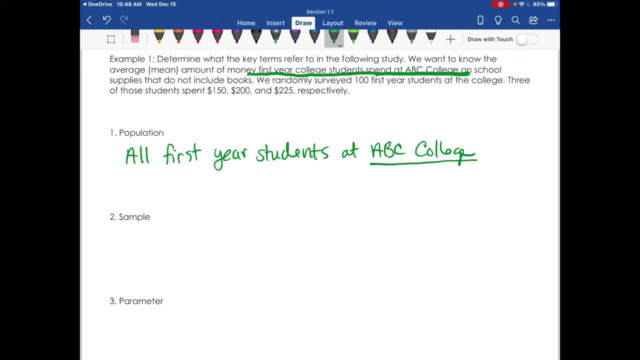 all first-year students either. You have to be very careful with the wording and make sure you underline the keywords so that you have all the information. So the sample is how we're going to collect our data. It's going to be very difficult. 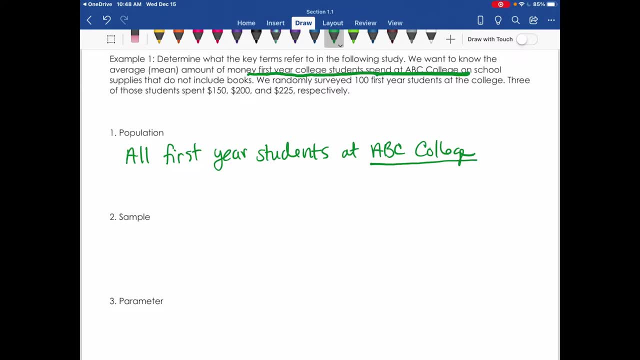 for us to collect the information from all of this. We're going to collect all first-year students at this college, So we collect a sample And from that sample we gather the information. Now it says in this problem that we randomly. 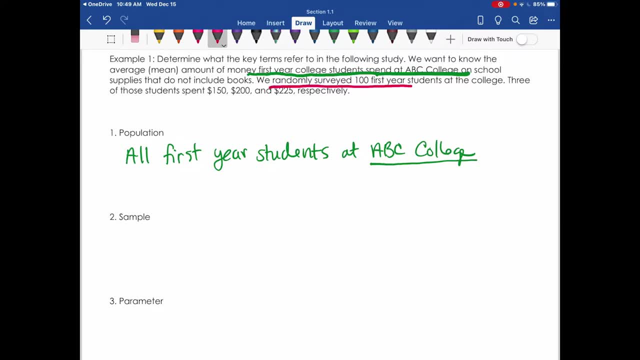 let me put this in a different color. we randomly surveyed 100 first-year students at the college, So that's going to be the sample. That's where they collected. the information is from those 100 first-year students at the college. 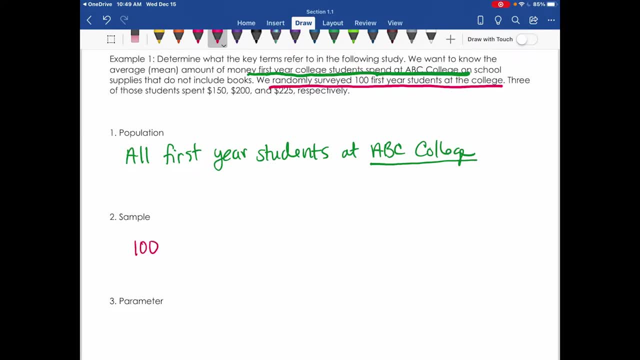 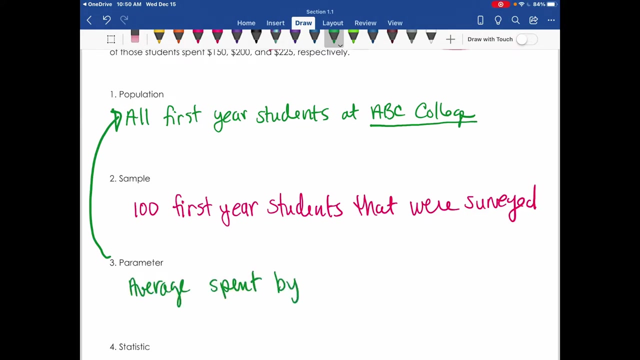 So let me put that down. So the 100 first-year students that were surveyed, That is going to be the sample. Then the parameter would be the average bench by first-year students At ABC College. Now, how did I know? 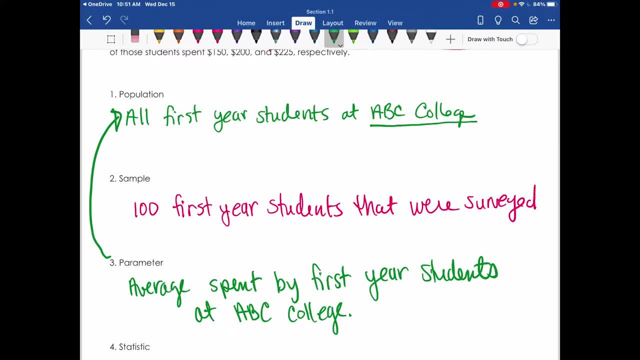 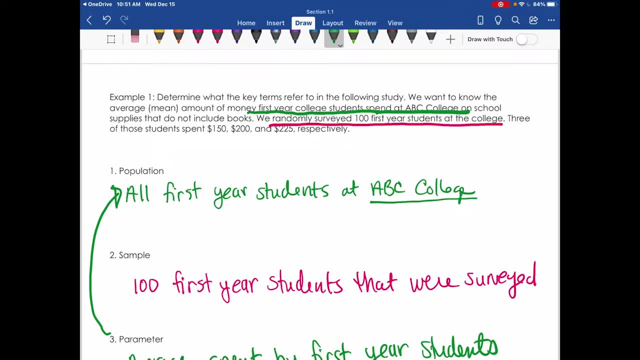 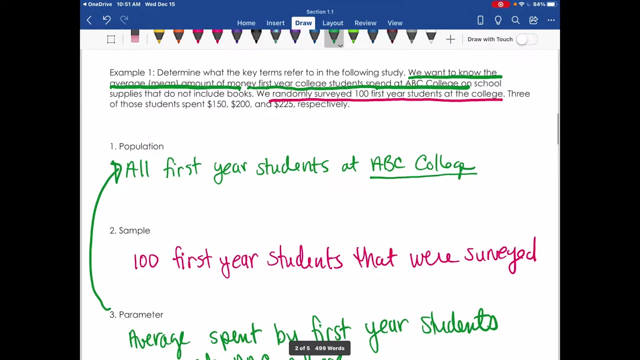 it wasn't a proportion Because, we said earlier, the parameter could be an average or a proportion. If we come up here and we read the question carefully, the question says what we want to know. We want to know the average amount of money that the first-year college students spend. 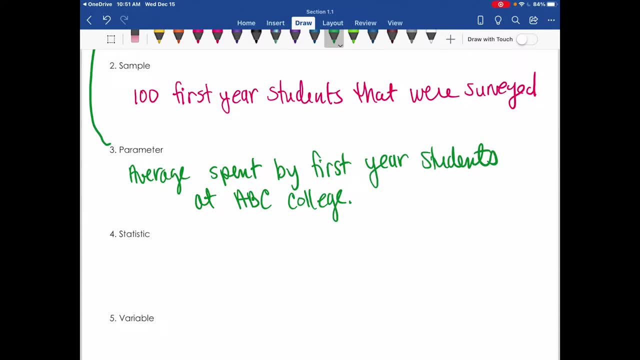 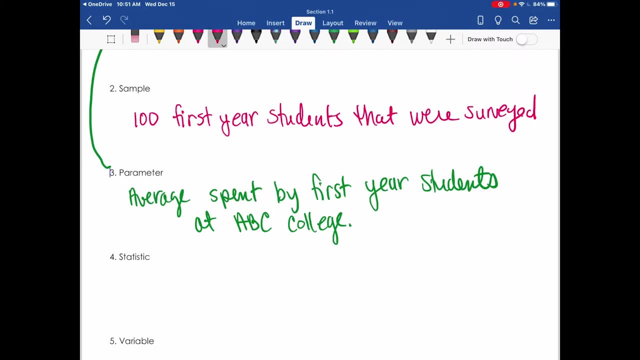 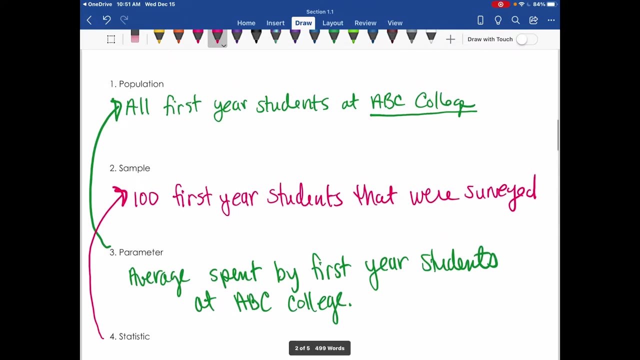 So if you want to make sure you're looking for the right parameter, go back and read the problem. It's going to be an average or a proportion. Now, remember, the statistic is calculated from the sample. Now, if you scroll back up, 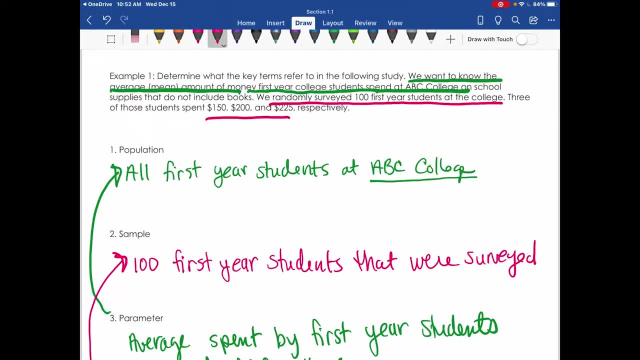 you'll notice that they give us some values here. They only give us three though. So if I take the average of 150,, 200, and 225,, that's not going to give me my statistic. My statistic is the average. 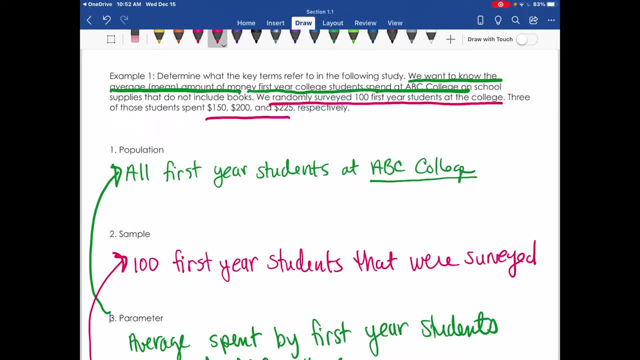 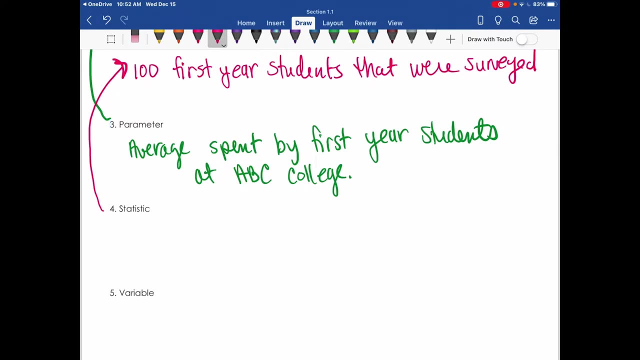 of the entire sample, And the entire sample consisted of 100 students. So if I use that average, it would not be the statistic. I want to make sure, even though they don't give us enough information for us to calculate it. 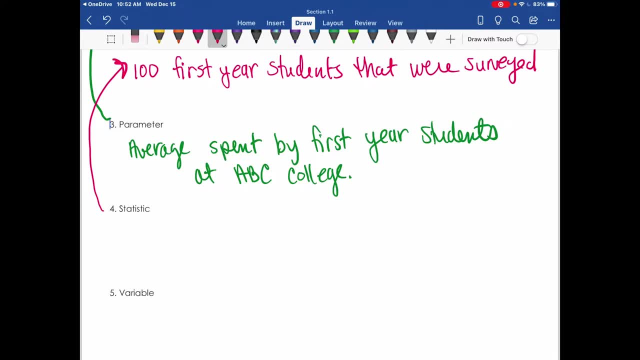 I want to make sure that I label it correctly. The statistic is going to be the average spent by the 100 students that were surveyed, So I'm going to put in parentheses the average of the sample. So the variable is what's going to change. 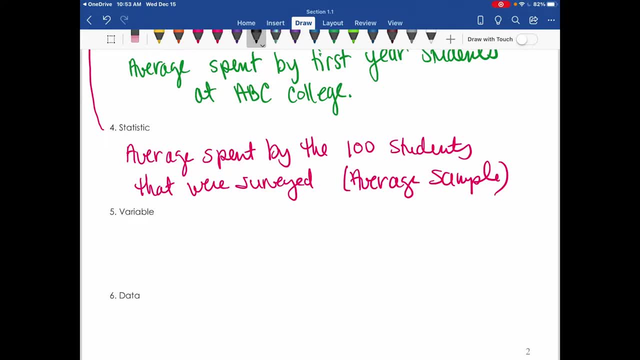 from student to student when I survey them. What am I trying to find out? I'm trying to find out the amount of money that the students have spent, omitting the cost of the textbook, but what they have spent on school supplies. So when I go to the first student, 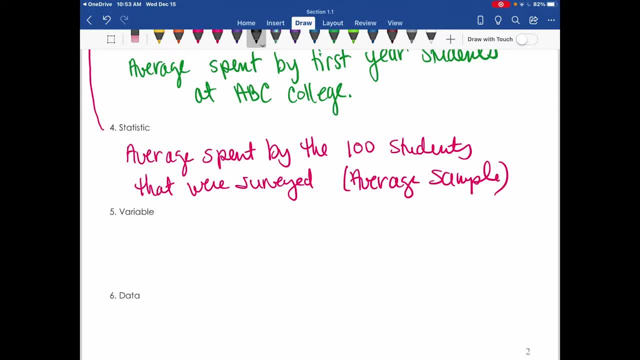 he's going to give me one amount. When I go to a different student, they're going to give me a different amount. So what's changing from student to student when I approach them and survey them is going to be the money spent. 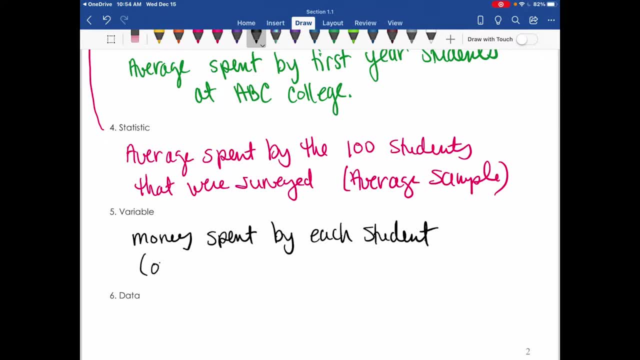 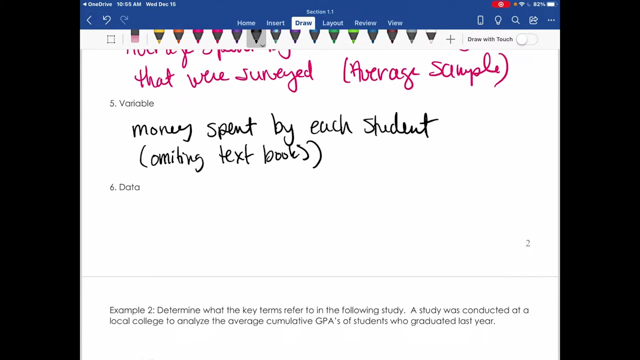 Okay, and then I want to make sure this is omitting the textbook. That amount is not going to include the textbook cost. Okay, data is going to be all the dollar amounts spent by the first year students. That's what we're trying to collect. 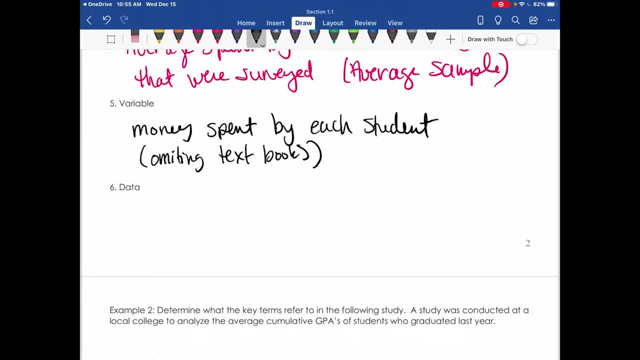 So when we collect that information, that's going to be the data. So this is going to be the dollar amount spent by the first year students. that has been collected, And these two go hand in hand. Whatever you're collecting, that's going to be your unknown. 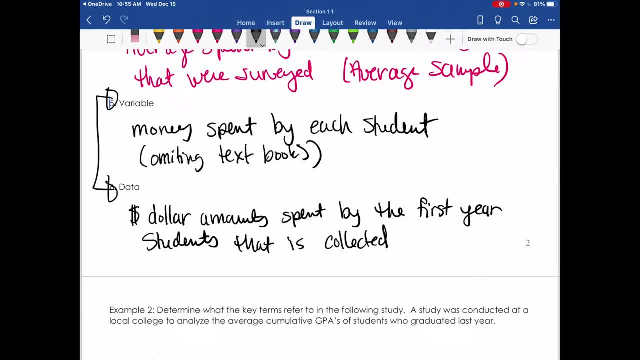 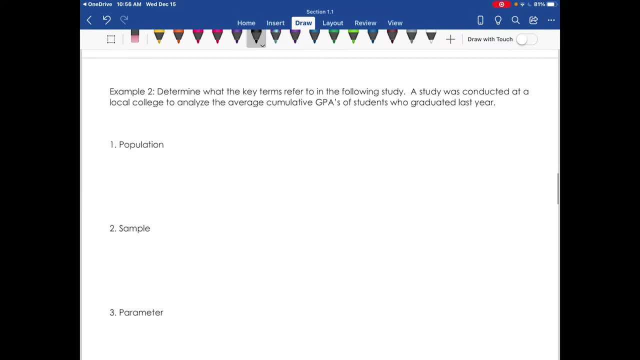 That's what you're trying to find out, And when you collect it, you're going to have those values And that's your data. Okay, let's look at example two. We're going to do the same thing. We're going to determine the key terms. 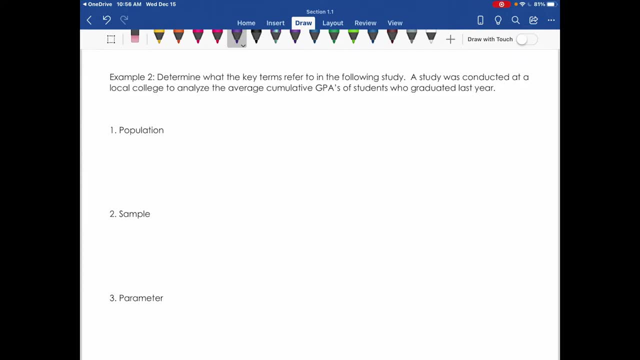 that refer to the following study. It says a study was conducted at a local college to analyze the average cumulative GPAs of students who graduated last year. So we are trying to find out about the average cumulative GPAs of students, But we're specifically doing it. 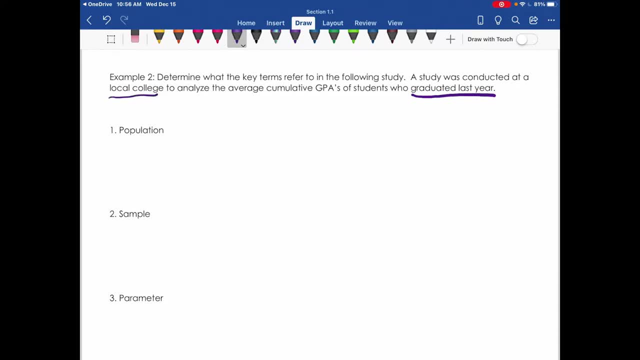 with the people that graduated last year from a specific local college. So we're not doing this for all college students. We're doing it specifically at this local college for the students that graduated last year. So our population where our focus of study. 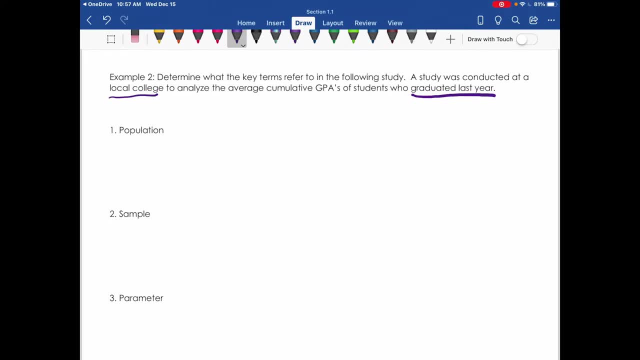 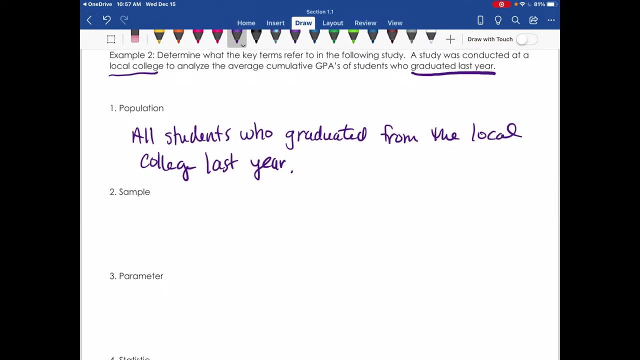 is going to be on the individuals or the objects that we're collecting the data from. this is going to be all students who graduated from the college, the local college, last year. Now we're trying to find or calculate the average cumulative GPAs. 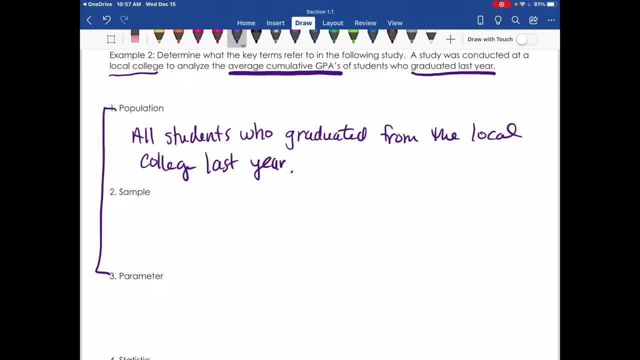 So if I had access to all those students and I was able to ask them what their cumulative GPA was and average them together, that would be the parameter. So the parameter I'll write down is the average cumulative GPA of students who graduated. 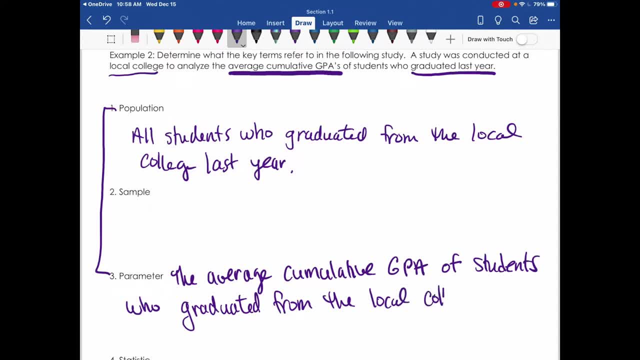 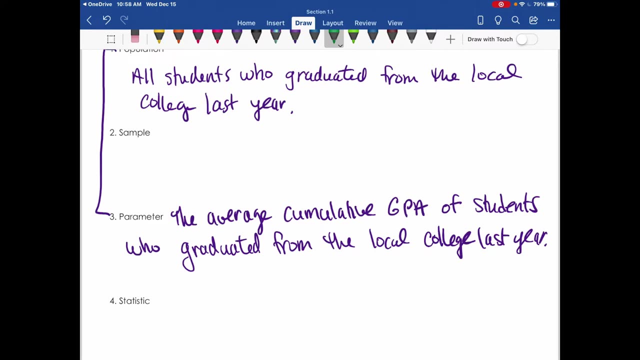 from the local college last year. Now the sample is going to be the students that they actually collect the information from. They don't give us the information on how it was collected or how many students they surveyed, So we're just going to have to state this. 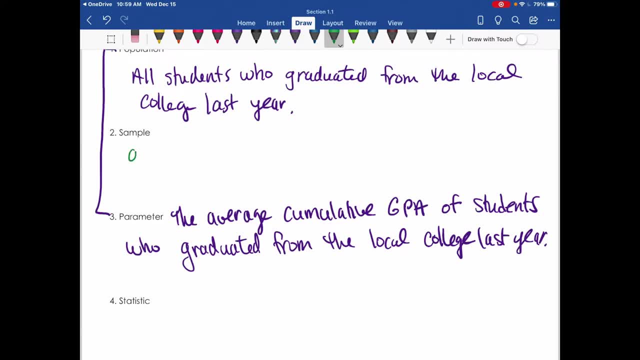 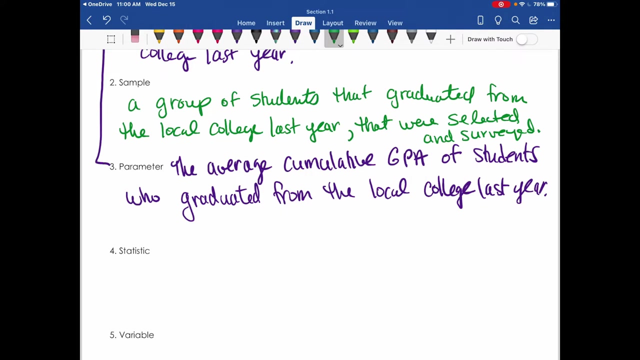 in a very generic way. So we can just write down a group of students, a group of students that graduated from the local college last year, that was selected and surveyed. Now, when they collect the information from that group and they calculate the average, 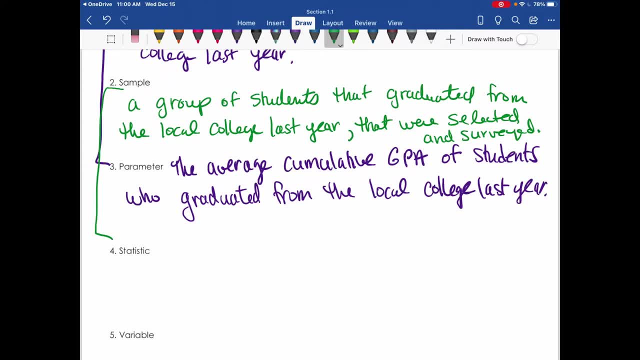 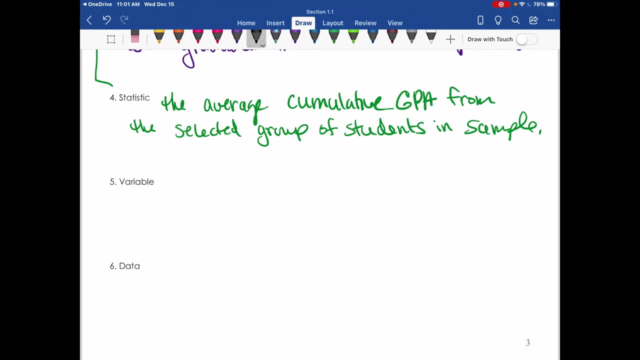 specifically from that group. that's going to give us our statistics. So our statistic is going to be the average cumulative GPA from the selected group of students in the sample. Now the variable is going to represent what changes from person to person when we're surveying. 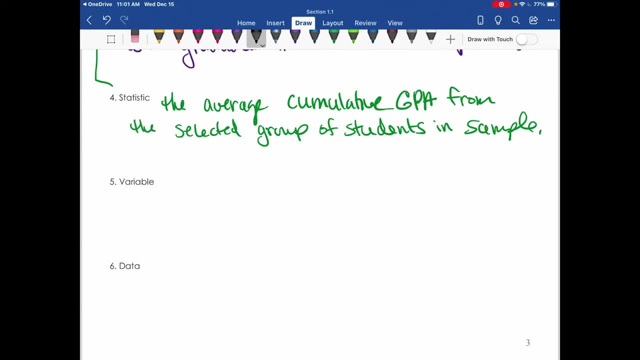 those students. So when we're surveying the student, one person is going to give us a GPA, Another person is going to give us another GPA. So the variable is going to represent the cumulative GPA given by the student. The data is going to be: 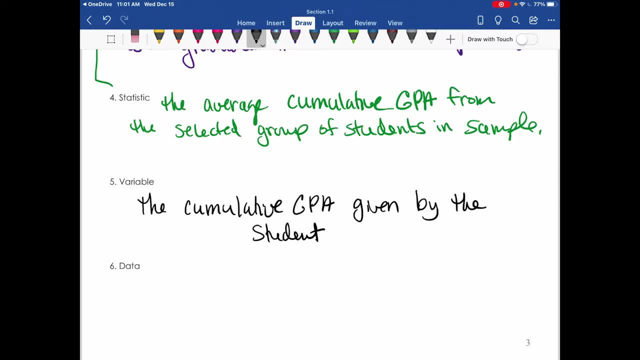 the set or the collection of all this information that was collected. It's the set of each of those cumulative GPAs that were collected, The set of GPAs- specifically- I'll put cumulative because I forgot that- that were collected from the students. 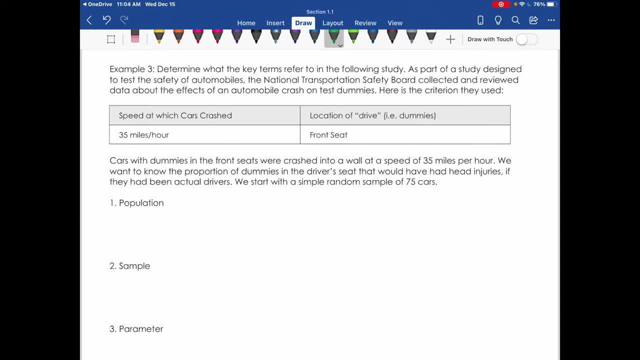 Okay, in example three, we're going to do the same thing and identify the key terms. that's related to the study And it says: as a part of a study designed to test the safety of automobiles, the National Transportation Safety Board collected and reviewed data. 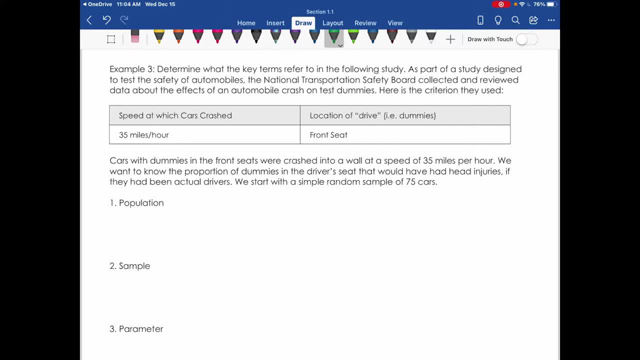 about the effects on the automobile crash on test dummies. Here is a criterion that they used. So the speed was 35 miles an hour for the car, and then the test dummies were put in the front seat. So cars with dummies. 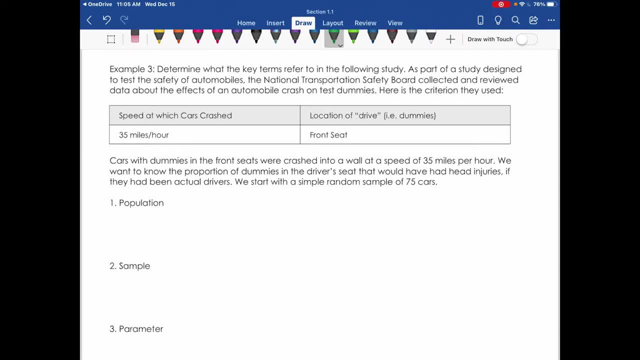 in the front seat were crashed into a wall at a speed of 35 miles an hour, And what we're trying to figure out is the proportion of dummies. I'm going to underline this because this is key words here: the proportion of dummies. 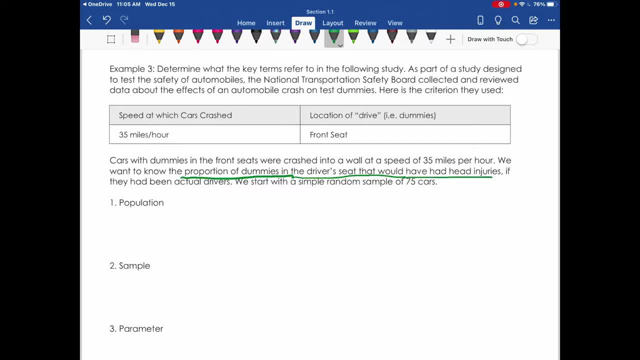 in the driver's seat. that would have had a head injury if they had been actual drivers. And we're going to have a random sample of 75 cars, So they do a ton of tests, 75 of those test cars, If you see. 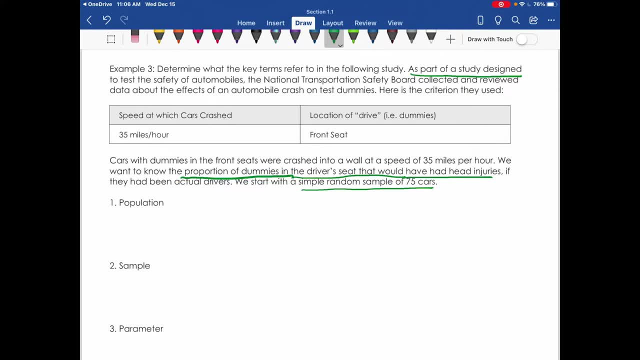 if you go back and look at some of this key wording, it says: the study is designed to test the safety of automobiles, So we're focused on the automobiles, The population is going to be all cars and we're going to study cars. 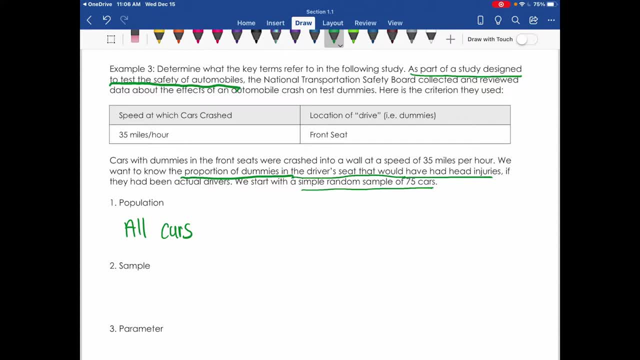 with the dummies in them. So I guess we could say with seated dummies, And I'll put in there specifically the front seat. Now the sample is going to be the 75 cars that were selected using a simple random sample. 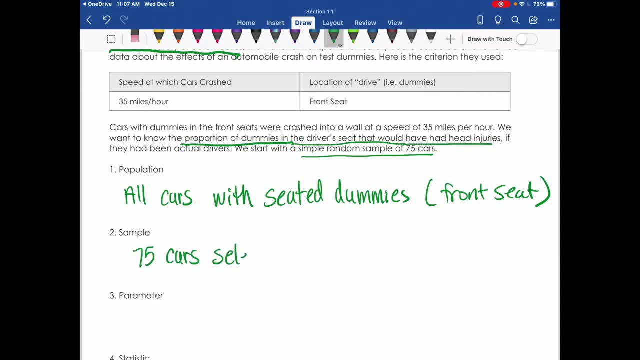 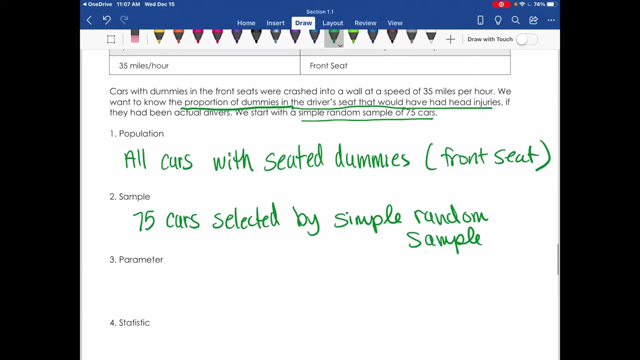 And they are going to be the 60 cars from the first day. Now, remember, the parameter is that value that we're trying to calculate And we want. the parameter is going to come from the population, So in this case, the parameter comes from the distance. 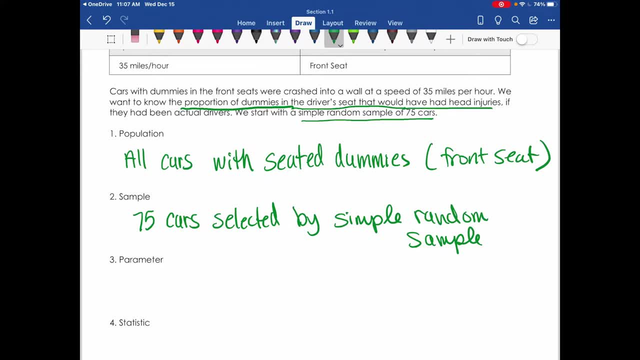 So in this example you're going to say it's the distance from the highway. that would be 70, case. the parameter is going to be a proportion and that's in here stated right here we're trying to find the proportion of dummies in the driver's. 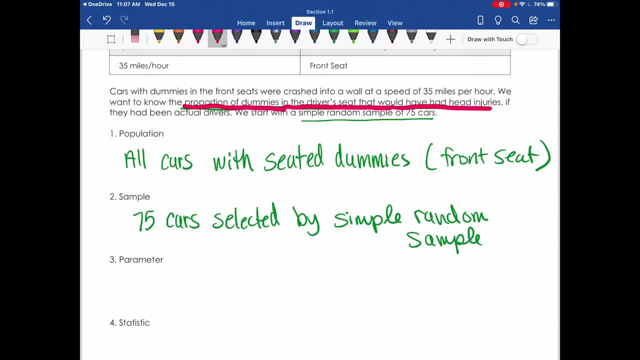 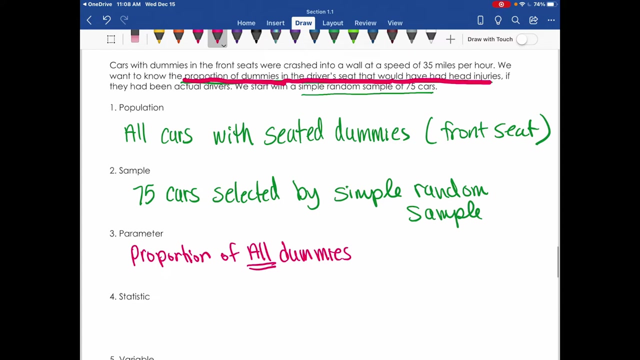 seat that would have had head injuries if they were an actual person. so we want to find for the parameter, since this is focused on the population, we want to find the proportion of all dummies. so all because this is coming from the population that would have sustained a. 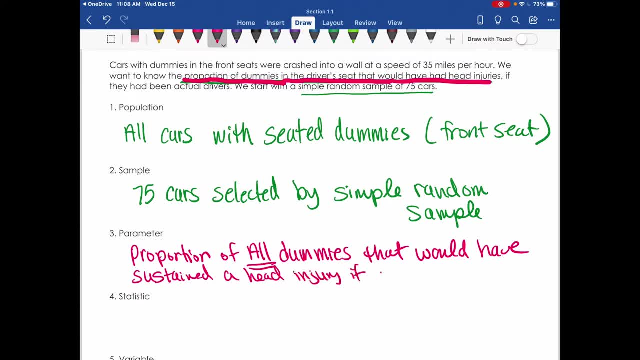 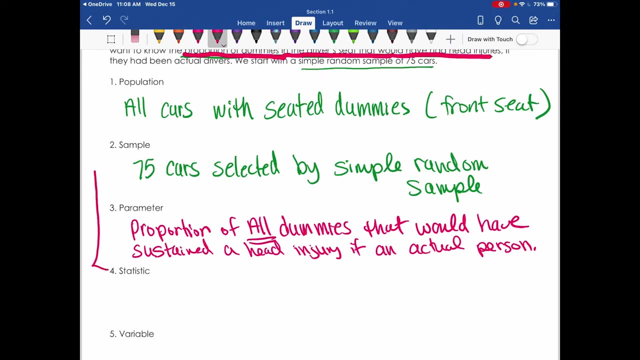 head injury if it was an actual person. person, the statistic is going to come from the sample, the parameter comes from the population. so everybody. the statistic comes from the sample, which is the group that's surveyed or checked. so the statistic is going to be the proportion of dummies from the sample of 75 selected that would sustain a head. 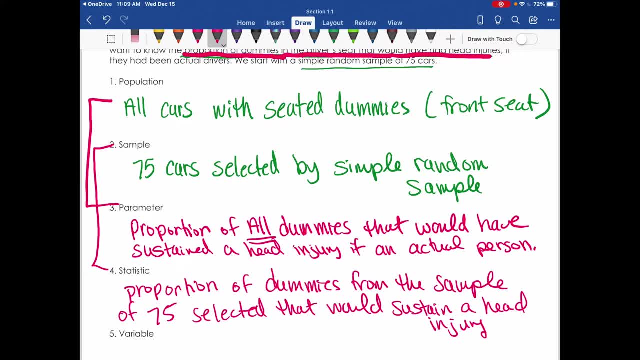 injury. so if so, let's say if 25 out of the 75 would have sustained a head injury if they were an actual person, my proportion would be 25 out of 75, which would be a third, or as a percentage would be 33.3%. so the variable here is going to be: 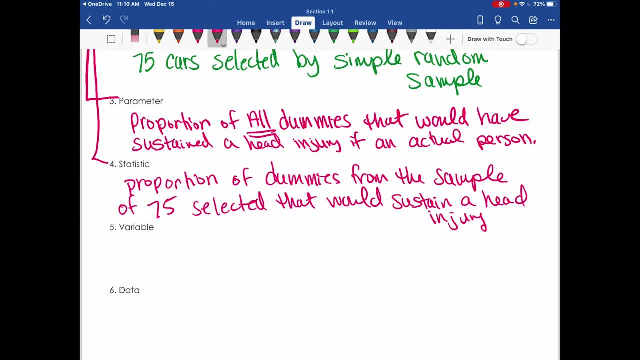 whether or not the dummy would have suffered a head injury if it was a real person. so when the 75 selected experiments were checked on, for each experiment you're going to have a different value. so when I look at one experiment, the first one, it's going to be a yes or no. 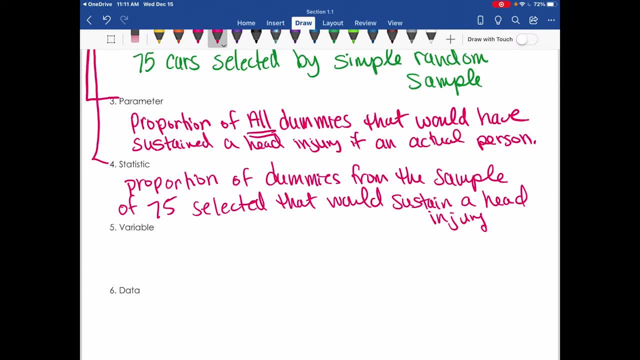 yes, they sustained a head injury or no, they didn't sustain a head injury. when i go to the next, when I go to the next experiment, it's going to be a yes or no. then i go to the next one, so what's changing? So what's changing when I check from each experiment to experiment? what's changing is whether or not the dummy sustains a head injury. 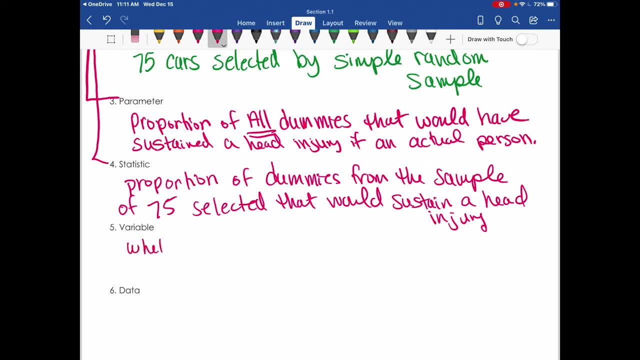 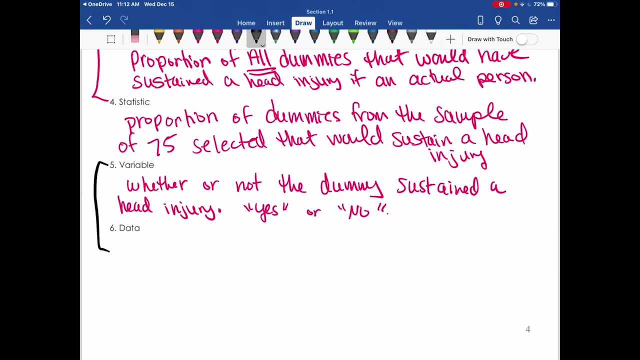 So the values that the variable in this case can take on is yes or no, or negative or positive, however you want to call it. So the data is going to be that collection of yeses and noes that I have. Okay, last example. 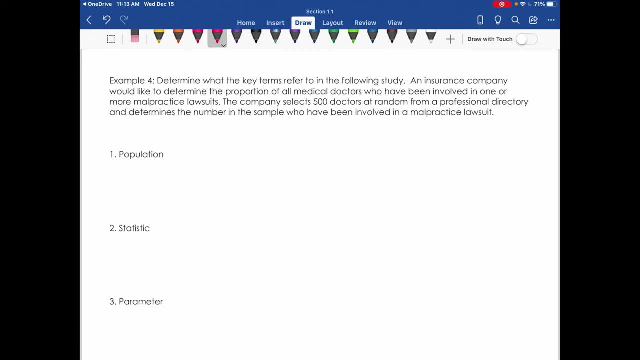 It says, determine what the key terms are that refer to the following study: An insurance company would like to determine the proportion of all all medical doctors who have been involved in one or more malpractice lawsuits. The company selects 500 doctors at random from a professional directory and determines the number. 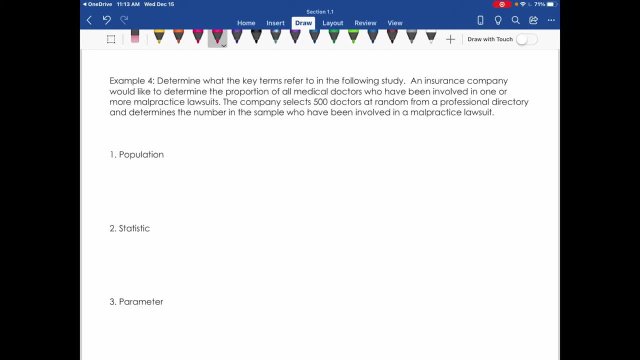 in the sample who have been involved in a medical malpractice lawsuit. So the population is the people or the objects that we're focused on and where we're going to collect the data from. Okay, so We wouldn't say, in this case, all doctors, because when we collected the information, 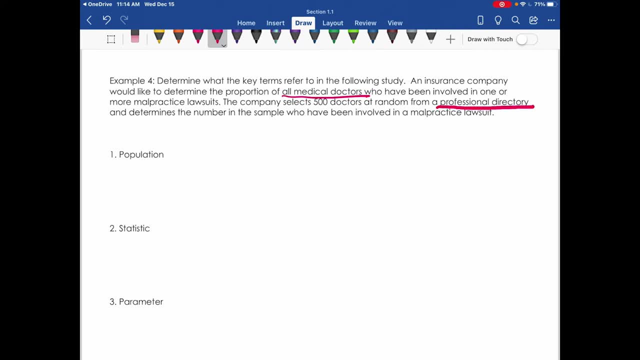 we collected the information from a professional directory. So if I said my population was all medical doctors and I only collected the information from one professional directory, that would not be a representative Sample, because I would need to make sure that I pick doctors from all different directories. 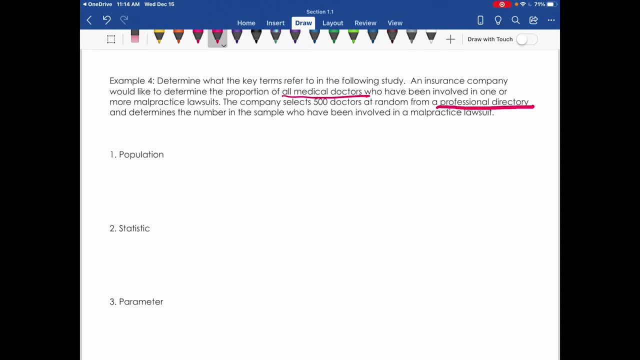 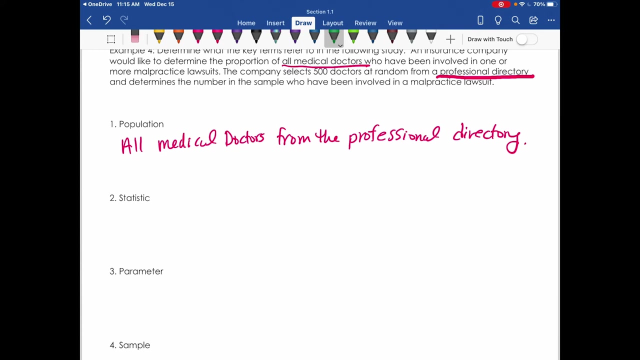 and all different areas, Because I'm specifically picking medical doctors from this professional directory. that is my population, So all medical doctors from the professional directory, So I'm going to pick doctors from this professional directory. Let's do sample next. So the sample is going to be the subset or the group that we choose from to collect the data. 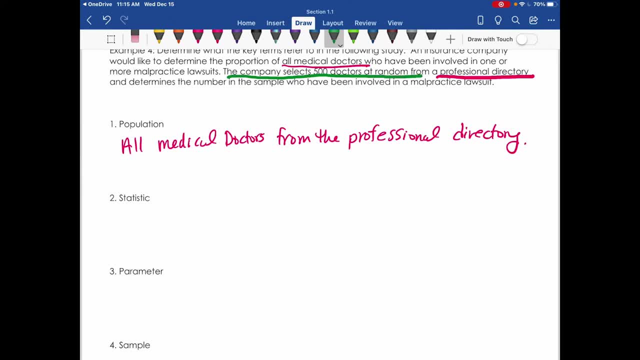 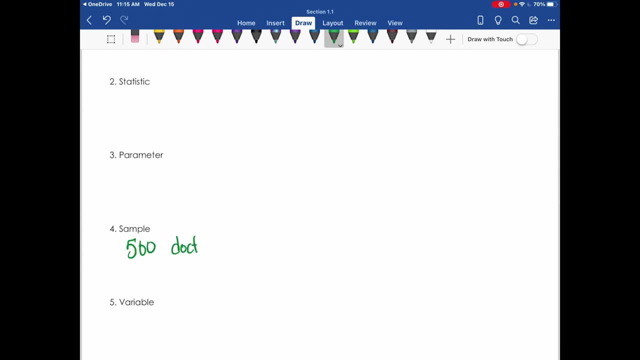 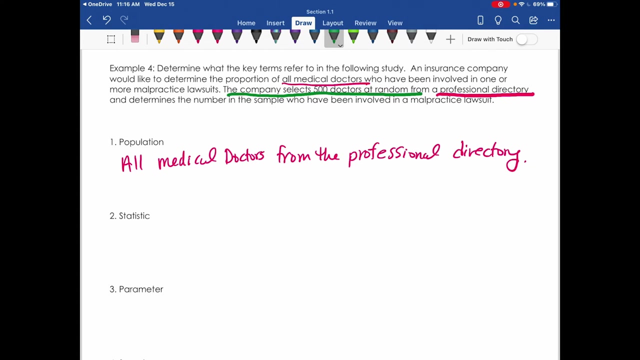 So it says the company selects 500 doctors from this professional directory. So the sample is going to be the 500 doctors picked from this professional directory. Okay, So The sample is going to be the sample that gets picked from the directory. Now the parameter is a value that is coming from the population. 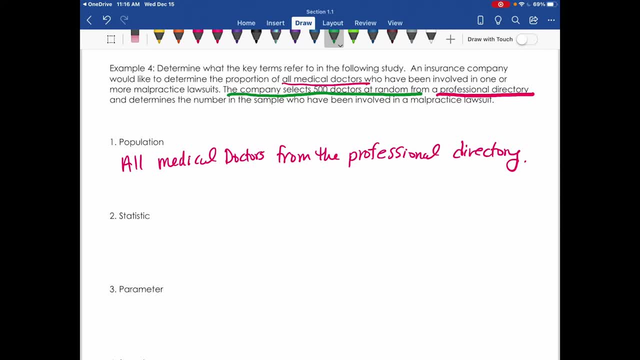 If I had access to the entire population and I make some kind of calculation based on every person in that population, that would be a parameter. When I look at the problem, it gives me a key word right here: proportion. Okay, a proportion of all the medical doctors that have been involved in one or more medical 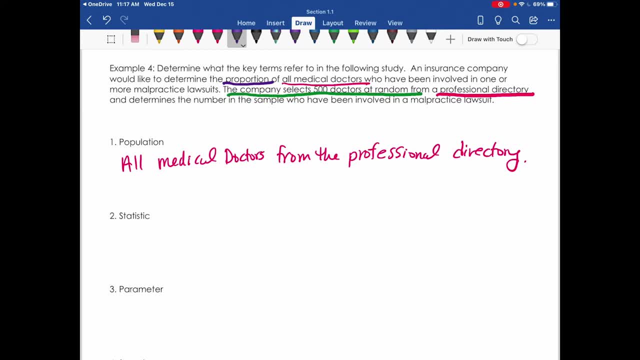 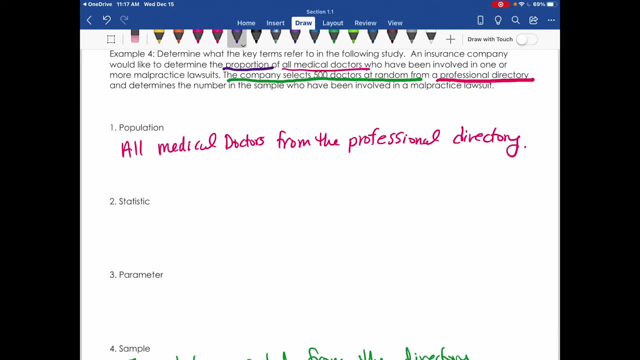 malpractice lawsuits. So, whatever that proportion is from the entire population, that is going to be my parameter. It's the proportion of all medical doctors from this directory that was involved in at least one malpractice lawsuit. So this is going to represent either a decimal, a fraction. 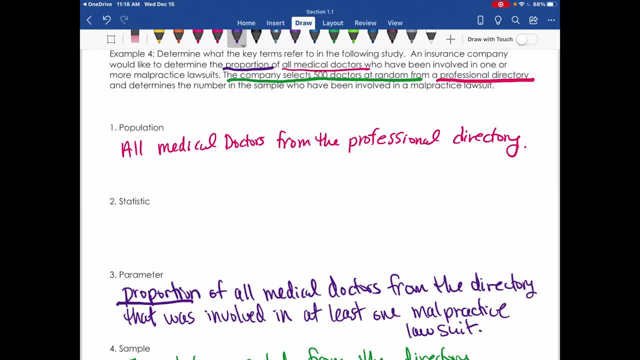 or a percentage of those doctors that were involved in a malpractice suit. if I was able to calculate that about the entire population Now, if I calculated the proportion based on the sample, then that would be the 3.5.. So if I calculated the proportion based on the sample, then that would be the 3.5..